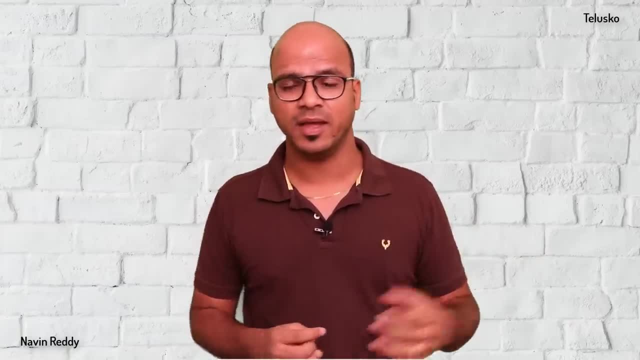 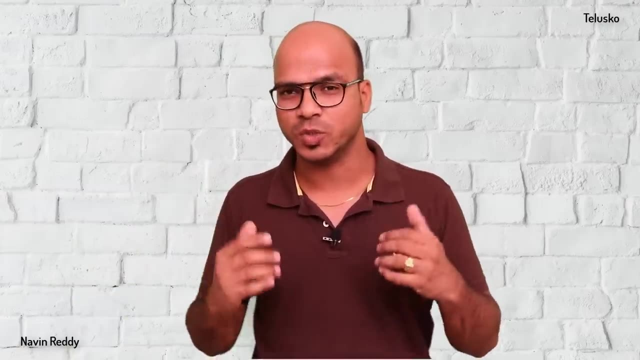 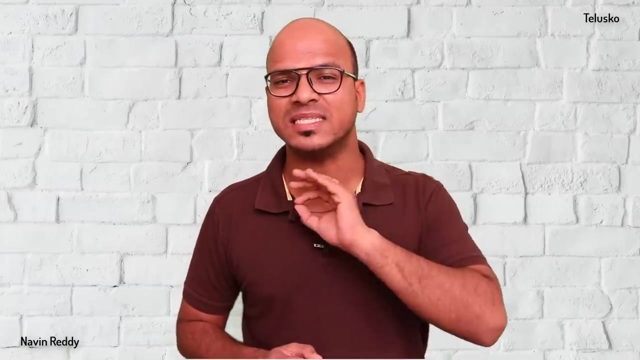 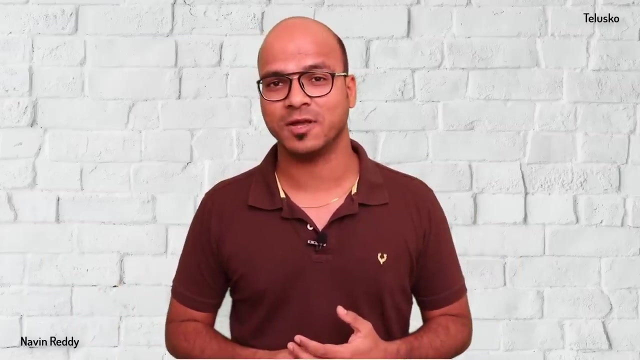 But now, since the advancement of machine learning, AI, this is a field where we have research scientists. they don't want to spend much time on learning programming language, So what they do, they went for the easiest language available. And the easiest language available in the market is Python. And yes, Python is damn easy. It is much simpler than C, C++ and Java. That's why most of the colleges and schools they are teaching Python. 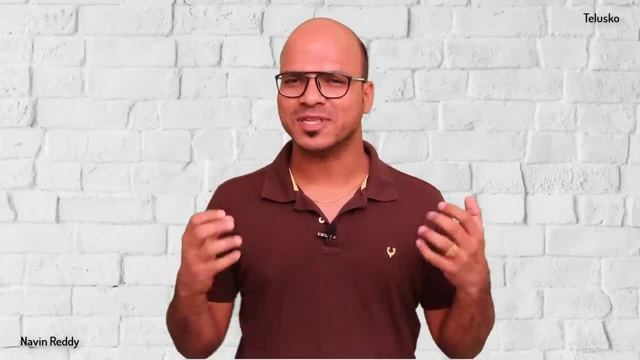 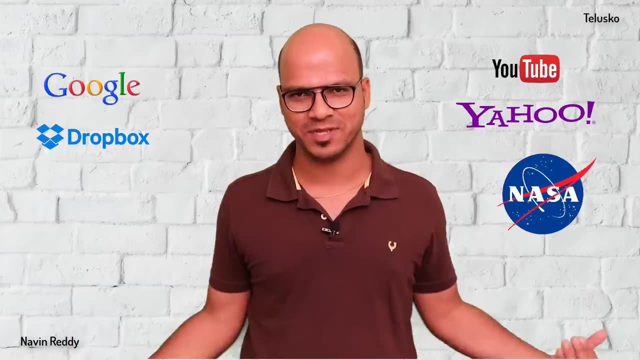 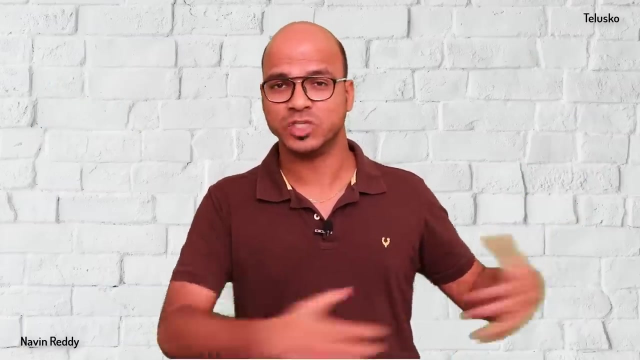 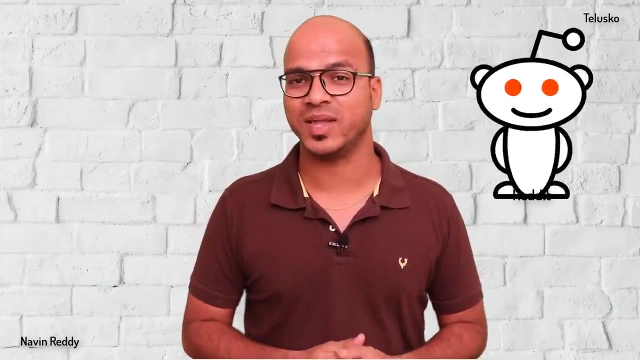 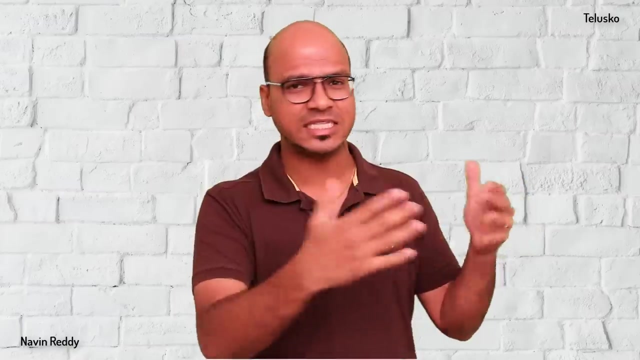 You might be thinking: which company uses Python? Now let's just list those small, small companies who uses Python. We have Google, we have YouTube, we have Dropbox, So we can see we have all these companies who are using Python as a main language or as a support language. Example: let's say Google has so many features. Some of those features is coded in Python. Now, in the same way, we have this one of the big website called Reddit. Reddit is today written in Python. Now let's focus on this name: Python. In fact, when you talk about C, C++, Java, these names, they have some story, right. 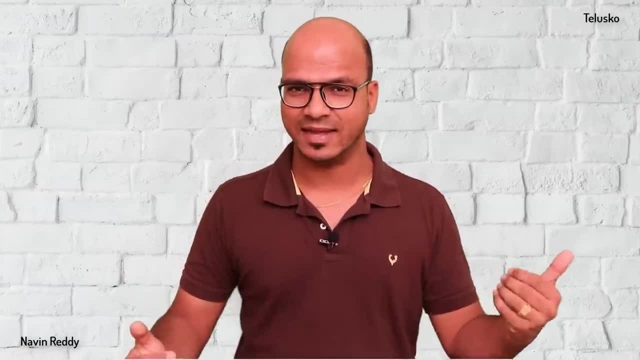 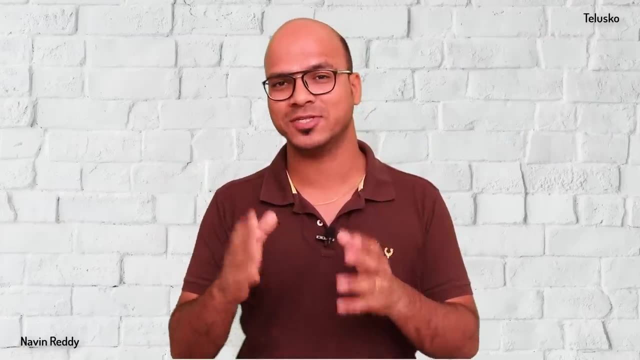 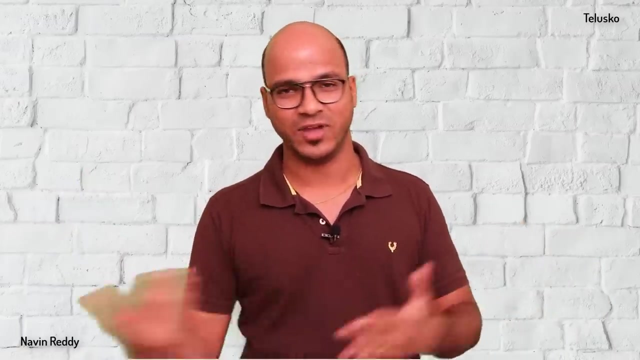 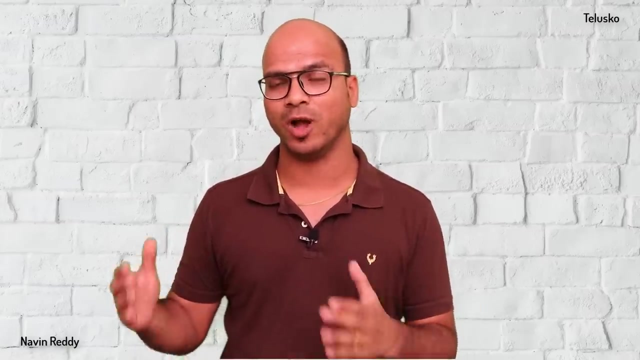 What about Python? It's just because this language looks like a snake, Not exactly The author of Python. he's a big fan of a British comedy movie called as Monty Python's Flying Circus, And that's why he went with a name called as Python initially, And then, when everyone wanted everyone liked it, he went for the same name. Now, can they learn Python? And the answer is yes. It is one of the easiest language to learn And even if you are from a non-technical background- you have not written any code- you can start with Python. What if I say Python k-4?? 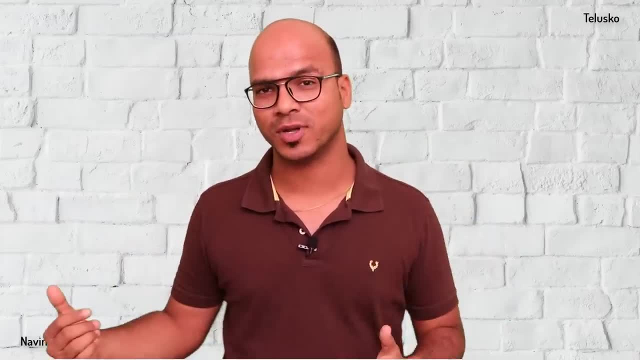 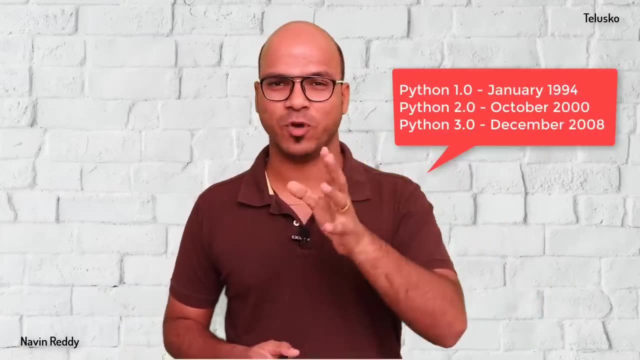 into picture, just to help those people who don't know how to add a code. in fact, children can learn python. it's that easy. now python has multiple versions. we have one point x, we have two point x and we have three point x, and of course, we should be learning three point x, right, that? 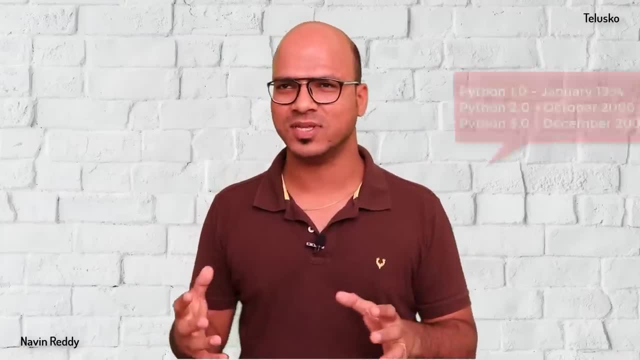 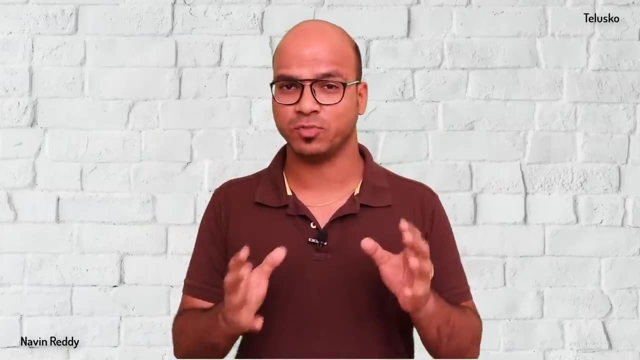 means two point x is not in the market and the answer is no, the mark the two point x is still in the market because when three point x came into picture, it was very different from two point x normally- what happens in programming language, you know. when java 8 came into picture. so it was. backward compatible with java 1.7. when job 1.7 came into picture, it was backward compatible with 1.6. but that's not the case with python. you know, the two different versions has two different way of working and that's why we have two point x still running in the market.